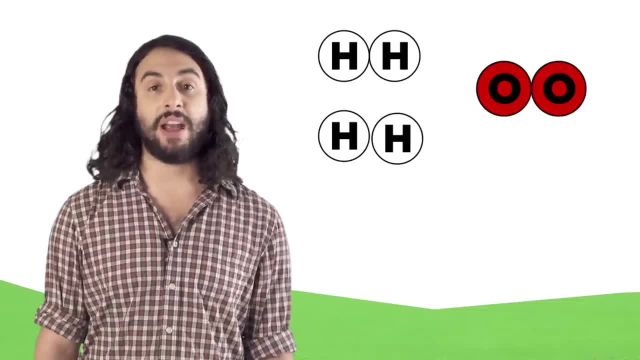 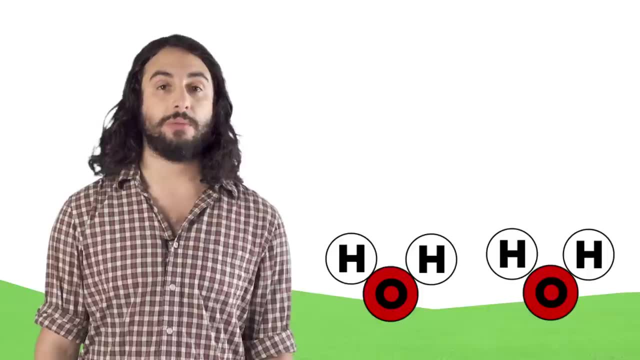 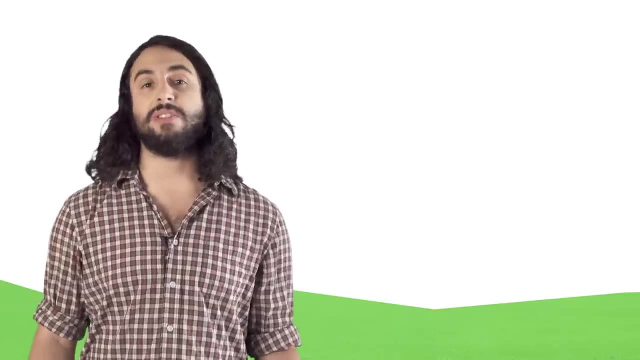 Here hydrogen gas and oxygen gas combine to form water. Notice that hydrogen and oxygen used to be connected to themselves and are now connected to each other. New bonds, new substance chemistry has occurred, So things like a substance changing from one phase to another are always physical changes. 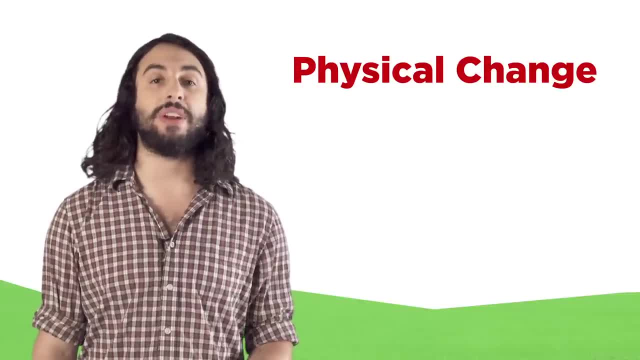 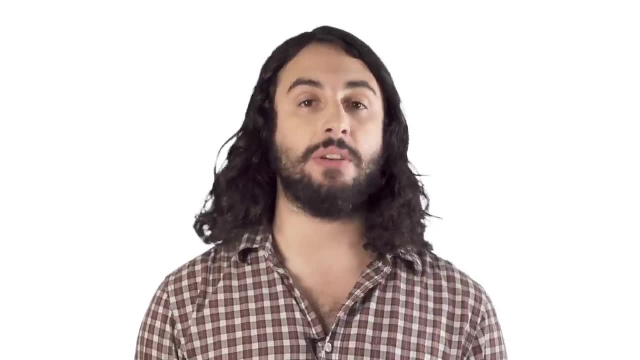 But if we make an entirely new substance with new chemical bonds, that's a chemical change. A pure substance is one that can't be separated into other materials by any physical process. Water: whether you boil or freeze, it will still be water. 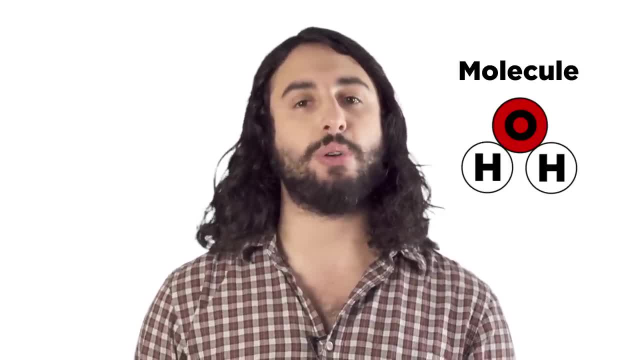 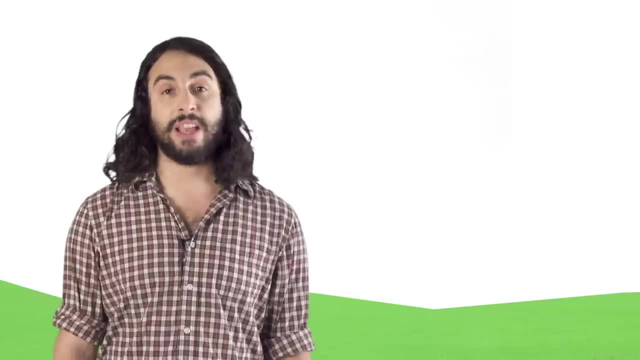 It's a type of molecule which is just multiple connected atoms. An element can't be broken down into smaller parts by physical or chemical means. For example, water is not an element, it's a compound, because it is made of two or more elements. 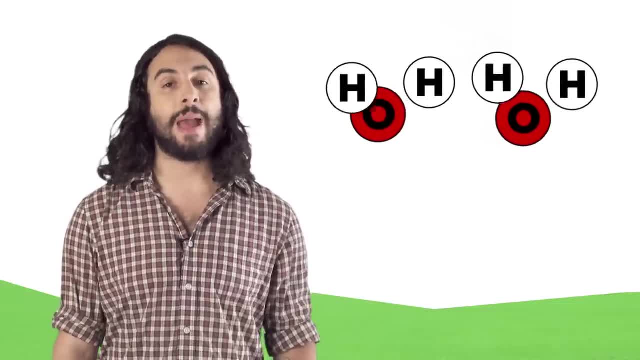 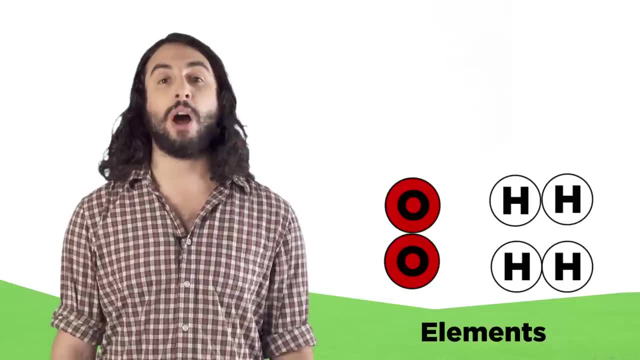 in this case oxygen and hydrogen. By a chemical process we can divide water into these two elements, but that's as far as we can go with chemistry. These are now molecules of a given element. A mixture is made of two or more pure substances. 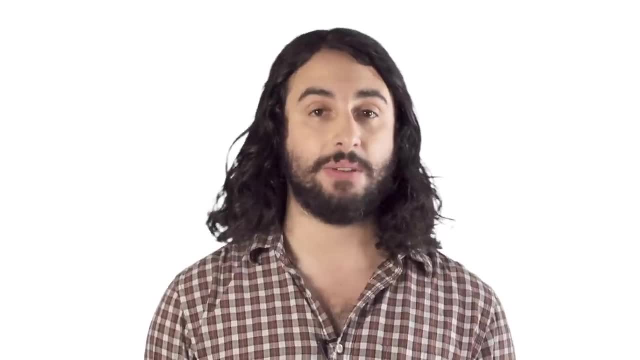 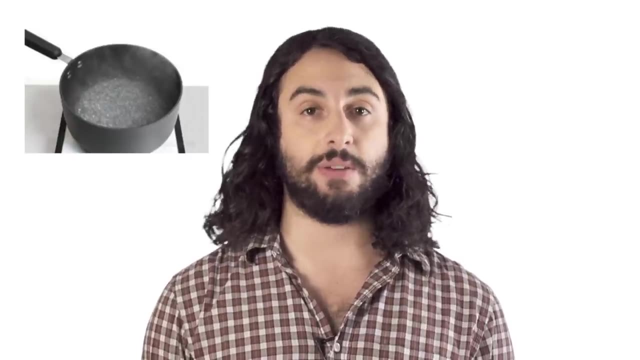 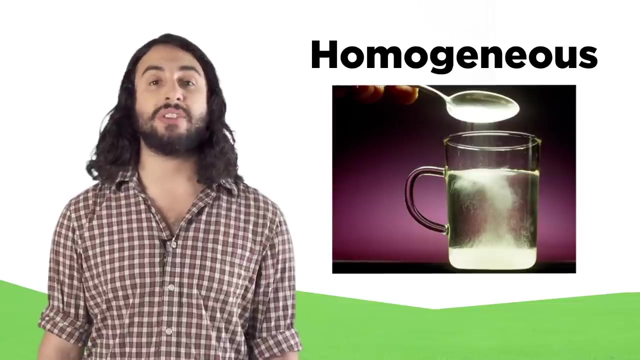 and these can be separated by physical processes. If you boil salt water, the water will evaporate and the salt won't, so the substances will have separated. A mixture can be homogeneous, meaning all the substances are distributed evenly and every section looks the same, like sugar and water. 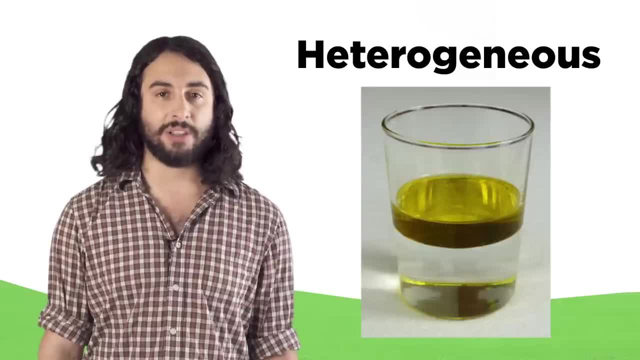 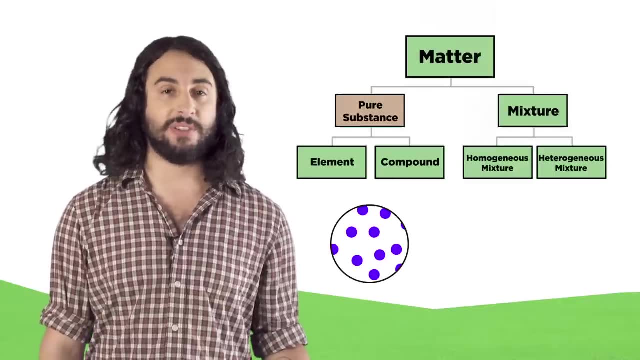 Or they can be heterogeneous, meaning they are not distributed evenly, and zooming in on different sections would look differently like oil and water. So we've got pure substances which can be elements made of only one type of atom. 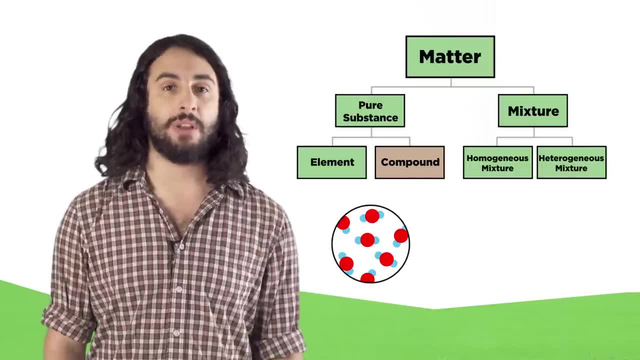 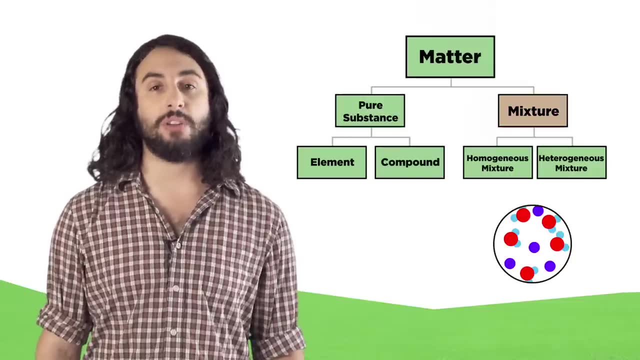 or compounds which are made of different types of atoms but are still just one type of molecule. Or we can have mixtures which are made of multiple types of molecules and are arranged in either homogeneous or heterogeneous fashion. Let's check comprehension.